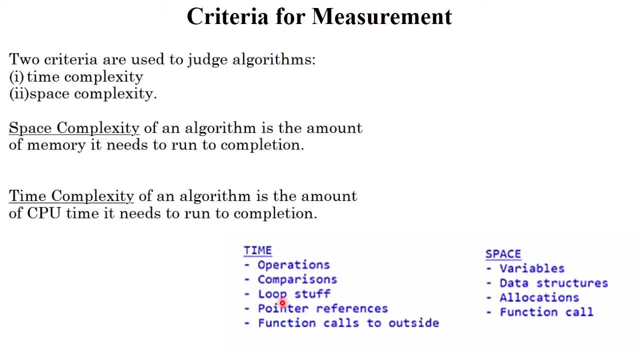 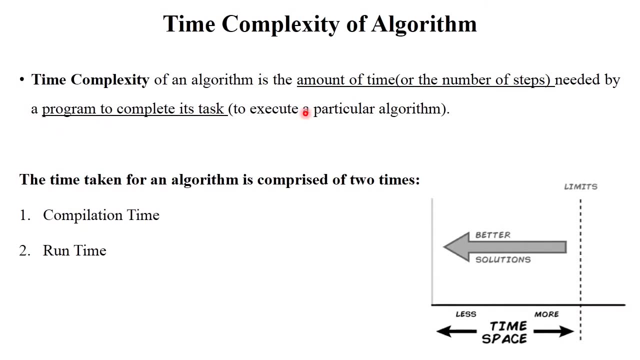 are performed in your program: The comparisons, loops, pointers and function calls to outside. These are the factors. Time is depend on those factors, Clear. So this is the concept of space and time complexity. Next Now time complexity of algorithm. What exactly mean time complexity, Time complexity of algorithm? 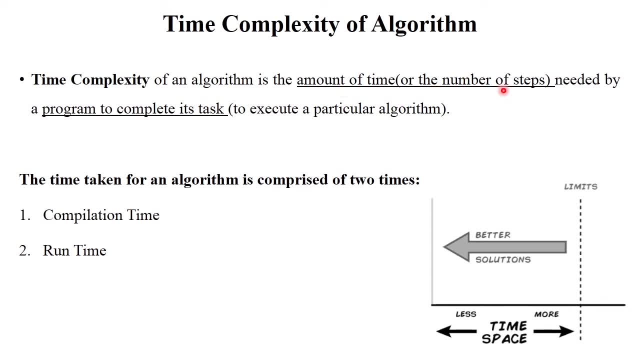 is amount of time. Amount of time depends on number of steps you have to perform in your program. Okay, So needed by the program to complete the task. To execute a particular program, how many times are required? This is called as time complexity, simply Okay. 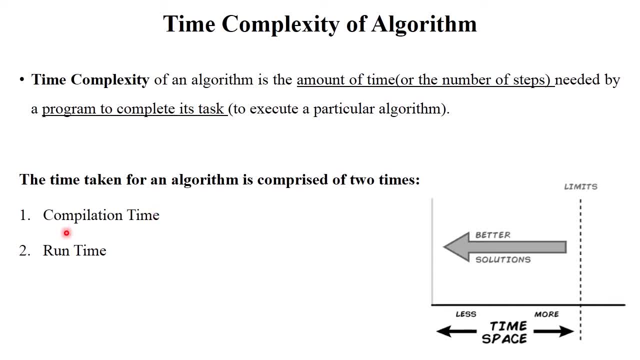 There are two types Of time complexity. One is compilation time and another one is run time. See in this diagram: If your program required less time and space complexity then it's provide a better solution, But it required a more time and space complexity than they have the limits It doesn't provide. 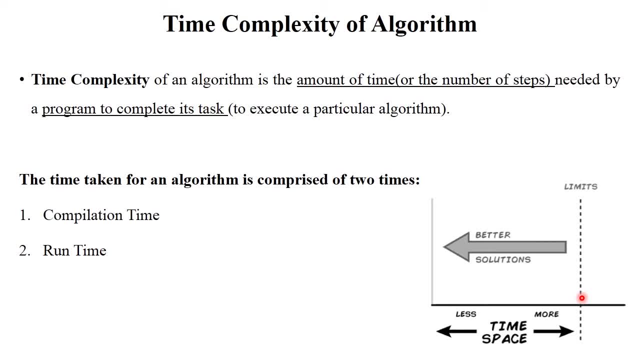 any better solution, Okay. So while implementation of program or while implementing a particular project, You have to always remember this thing: That's your project or your program required less time and space, complexity, Clear, So it provides the better solution, Okay. Next. 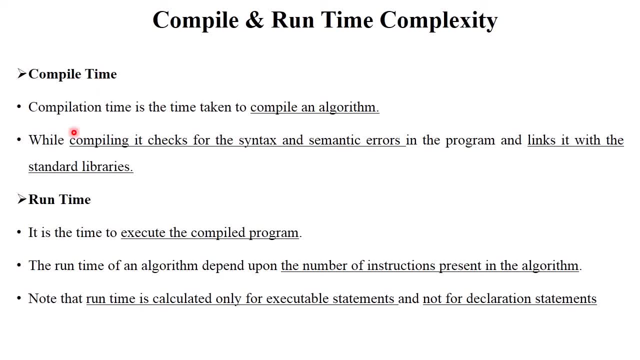 So there are two types of time complexity. One is compile time and another is run time. What is mean by compile time? So compilation time is the time taken to compile the program When you have to implement a particular program. So after implementation you have to compile. 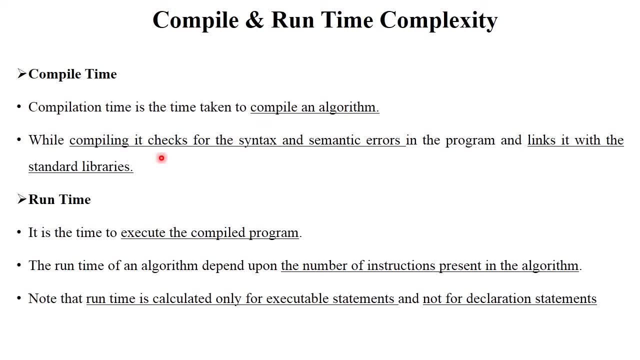 it by using some compiler or interpreter. While compiling it, check the syntax and semantic errors in the program. Syntax errors means they have the particular syntax, like if else switch case data types etc. So check the particular syntax in your program and semantic error. Semantic means meaning of each and every statement, Whether it is properly or. 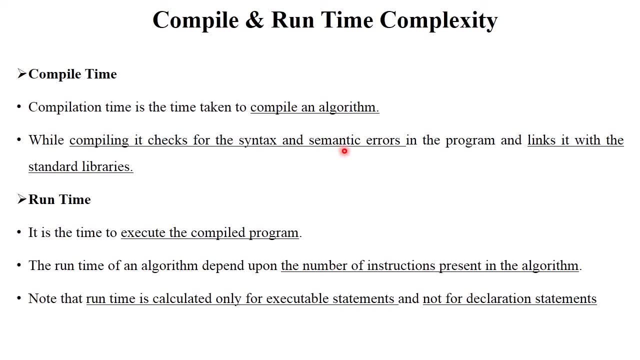 not. So compilation generates the syntax and semantic errors in your program And also sync it with the standard libraries. You have to use proper libraries or import library in your program. So compile time, check compilation, check all those syntax semantic errors and 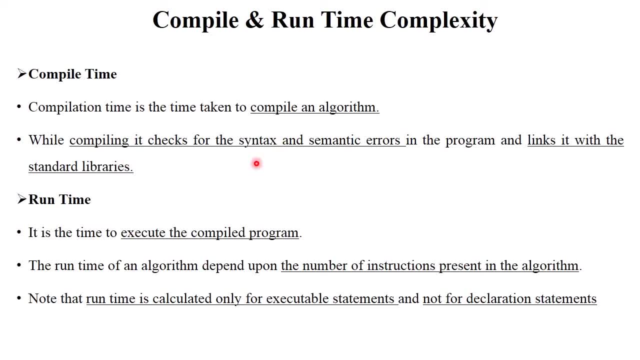 about detail library. So if there is any error, it shows the compile time error. Okay, So the time required for those analysis is called as compile time Clear, And the next one is run time. It is the time to execute the compiled program. 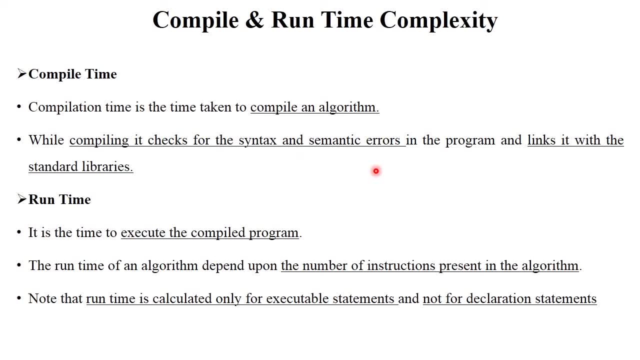 Okay, After compilation and after solving all the errors, you have to run your program. So this is called as execution. Okay, So run time algorithm depends on number of instructions present in the algorithm. Always use minimum instruction while solving the particular problem or while implementation of algorithm. Note that run time is calculated only for executable. 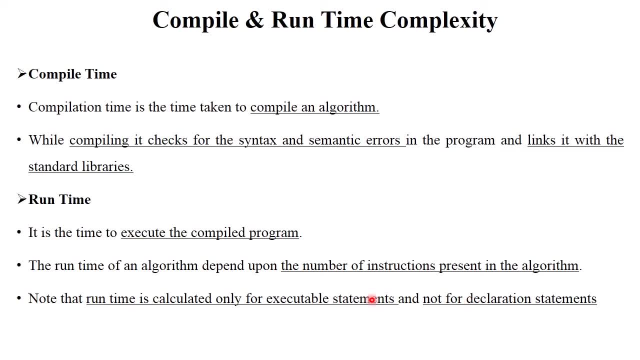 statements, Not for declaration statements. Executable statement means you have to use for loop, while loop, switch case, This kind of executable statements in your program, So run time depends on that Clear. So these are the two types of time complexity: Compile time means while compilation and run time. 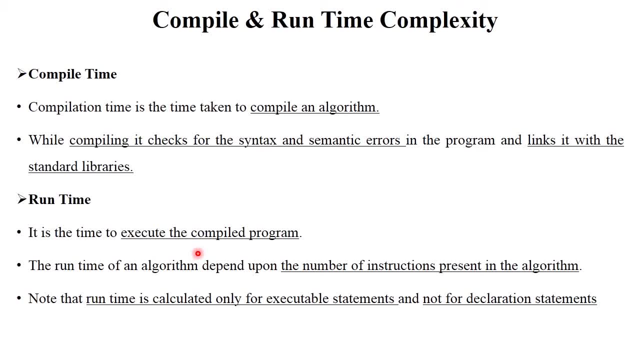 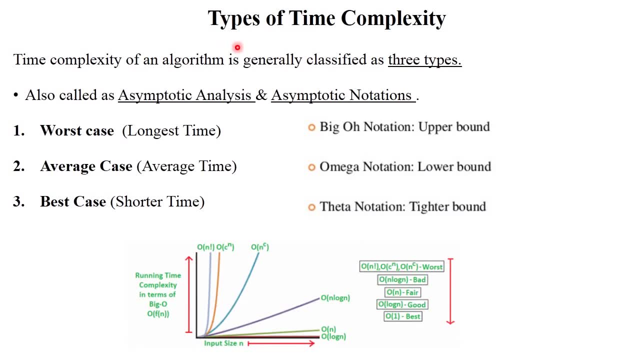 means after compiling program, at the time of run or implementation or execution of program. Clear. Next Now the next one is types of time complexity. Time complexity of algorithm is generally classified into three types, That is, worst case, average case and best case. So this is. 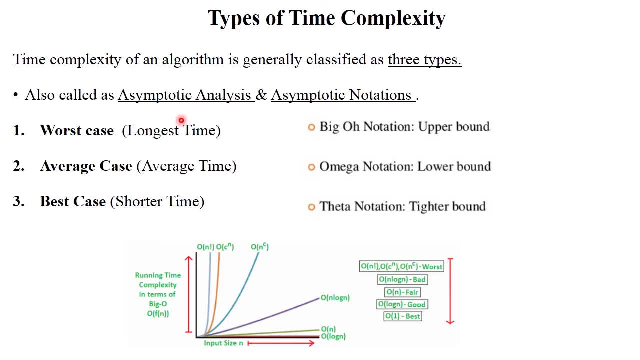 also called as asymptotic analysis. So what is mean by asymptotic analysis? What is mean by asymptotic notation? I will explain in detail in my next video. Okay, So in this video you have to just remember about these three things. there is three cases: worst, average and best case. worst case: calculate the longest time. 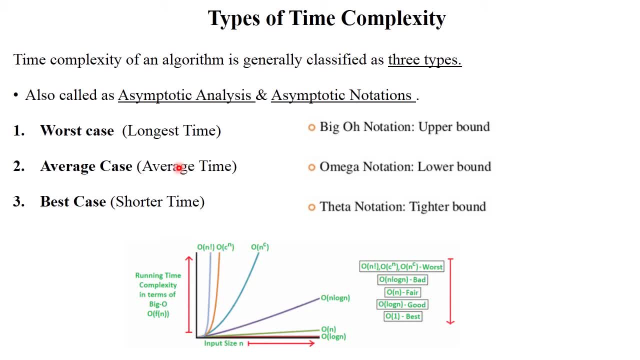 of your algorithm. average case calculation denote average time required to the algorithm and best case means shorter or minimum time for execution of your algorithm. okay, so this worst case is denoted by big O notation, average case denoted by omega notation and best case denoted by theta notation. so what exactly this notations are denoted, I will explain in next, my next video. 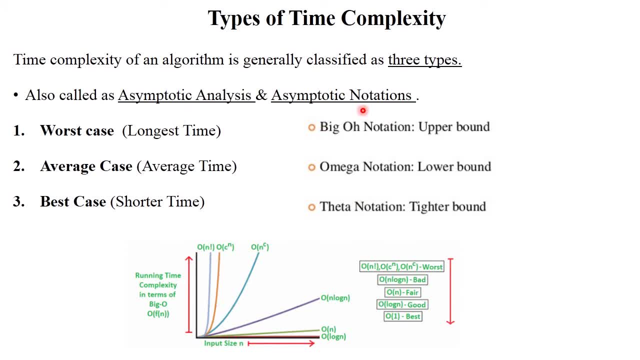 that is, asymptotic analysis and asymptotic notation. clear see in. in general life we have to use liter, centimeter, kilometer, right this kind of notations. so while measuring the complexity of algorithm, you have to use this notations: big O, omega and theta- clear you. 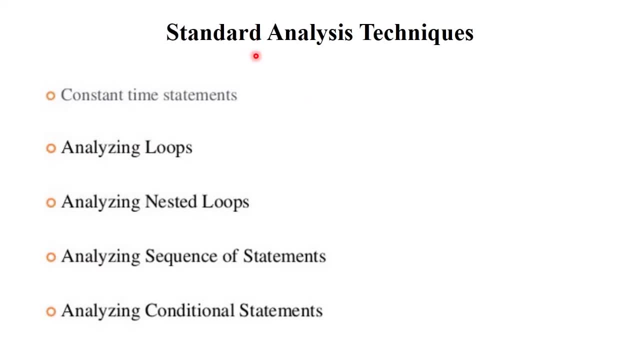 next, there are some standard analysis technique. the time complexity and space complexity are measured by using this standard analysis technique. you it analyze the loops in your program. constant time statements also analyze nested loop sequence of statements and conditional statements by analyzing all those statements in your program or in your algorithm. so time and space depend. 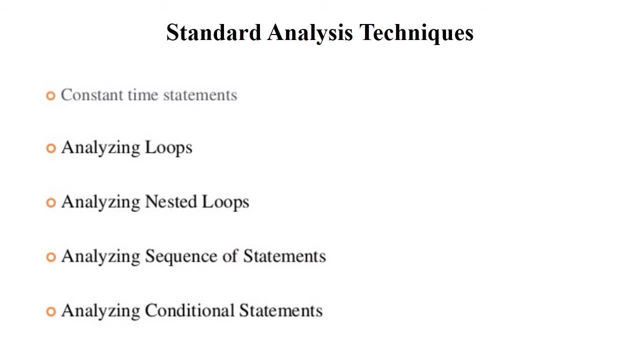 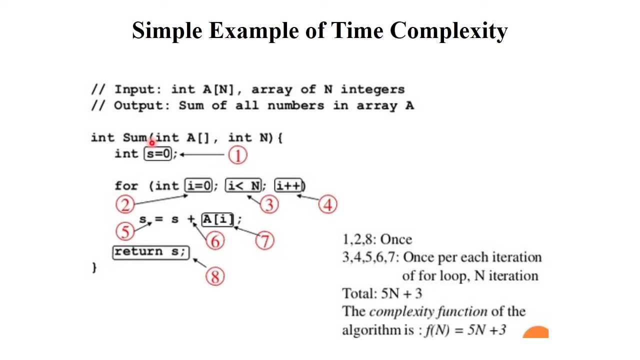 on those analysis: serious, clear. next, now here is a simple example of time complexity. okay, here, integer, we have passed to parameters like array and total number of elements. let it suppose and integer as equal to zero, you have to calculate addition. suppose you have to calculate addition of. 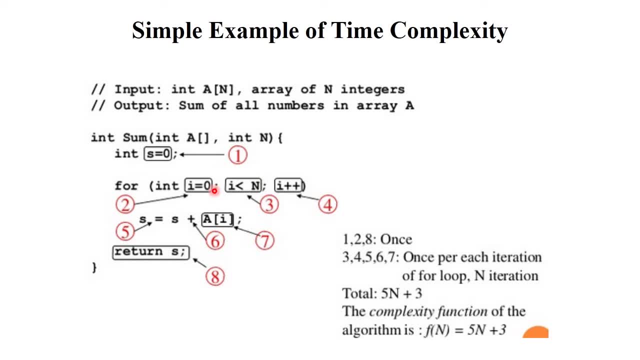 1 plus 2 plus 3. ok, I equal to zero, I less than equal to a. suppose we consider n equal to three. okay, pity god, all of them give idea here: integer sum of numbers around the Plan for a total number. z has to be something here. you have to 我. t colon스� sees integral of r equal to: 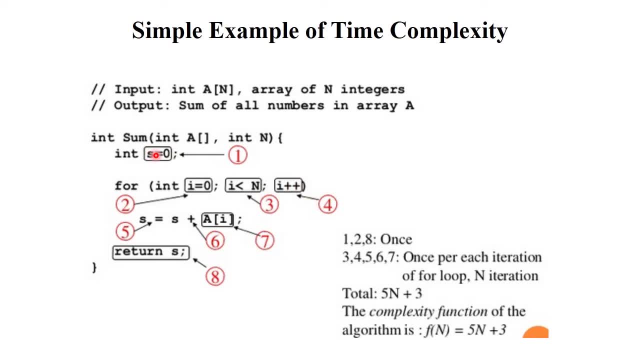 1 plus 2, and then you have the muss n as x, and since the rational of this proved on this and i++, So first value of s equal to 0.. 0 plus 1, 1.. Now value of s equal to 1.. Now it is s equal. 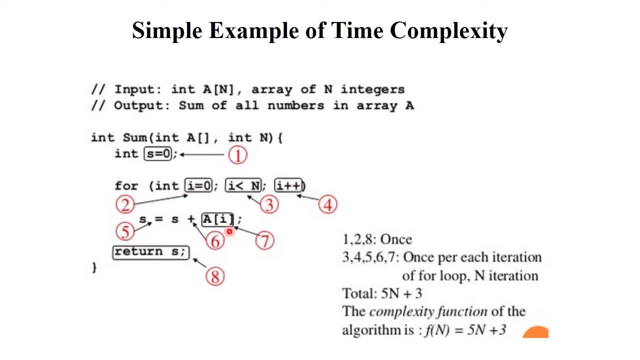 to 1.. It is i++, So after 1, it becomes 2.. So 1 plus 2,, 3 in this way. okay, Now see here The s equal to 0,. this is constant value. okay, That is fixed value. i equal to 0, again has constant. 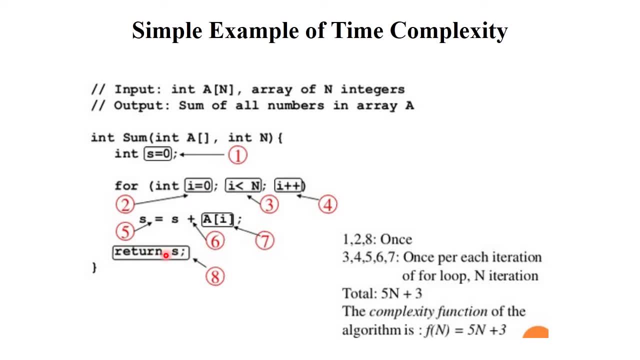 value and return s. Return s means final result. it can be written okay. So 1,, 2 and 8, these are the constant value or once value, right, And after that i less than equal to n 3, it generate the. 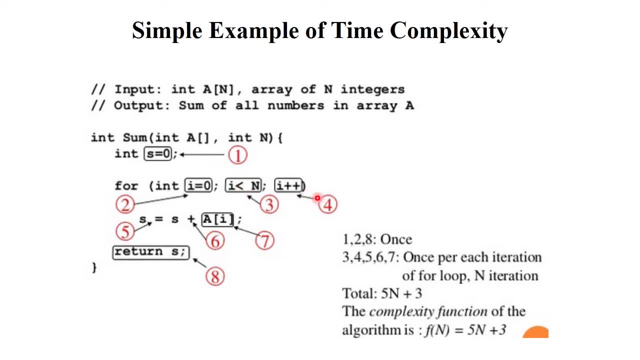 comparisons. These are not constant. okay, i++. these are also not constant value, continuously increment or variable part. okay, So 3, 4, then 5.. 5 means equal to Every time it can be calculate or addition is performed and stored value into this part. So 3,, 4,, 5, 6, 7,. 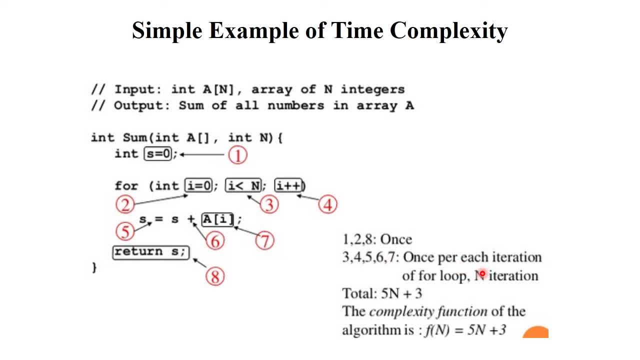 these are the variable part. So once per each iterations or for loop, there are total n iterations are required, clear. So how many constant value 3. And how many variable parts value 5.. So 5. And how many times it requires to perform the operation. That is n time, okay. 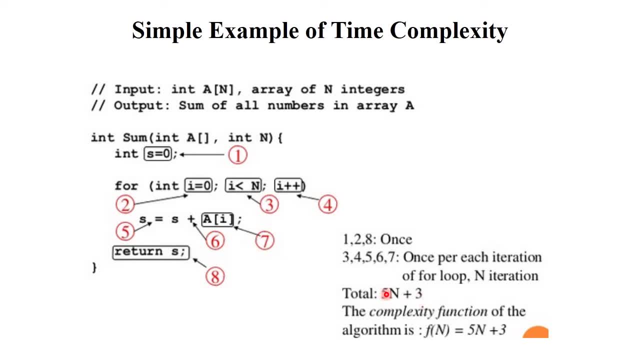 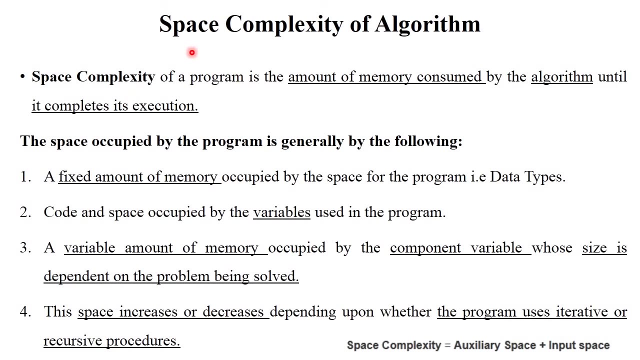 So 5 n plus 3.. These are the variable part and these are the constant part. So time complexity of function of algorithm is 5 n plus 3, clear, This is just simple example of time complexity. Next Now, what is meant by space complexity of algorithm? Space complexity of algorithm is: 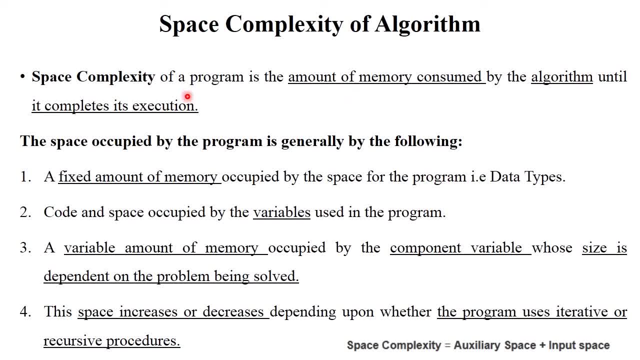 amount of memory consumed by the algorithm until it complete the execution? okay, How many types of how many memories required For the execution of particular program or particular algorithm? This is called as space complexity. The space occupied by the program is generally by the following ways: okay, So 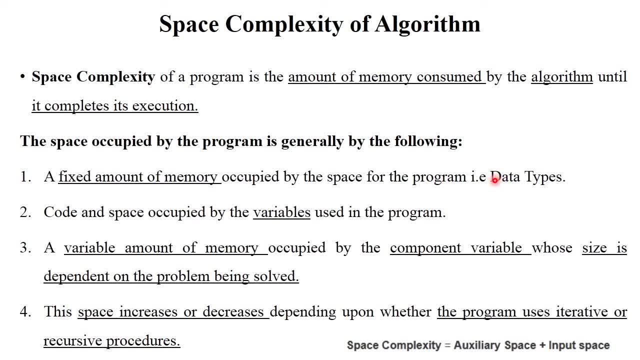 fixed amount of memory means some data types. Some data types require the fixed amount of memory. okay, So this is the one factor of space, complexity, Another code and space occupied by the variables used in the program. You have to declare integer a equal to 10.. So this a. 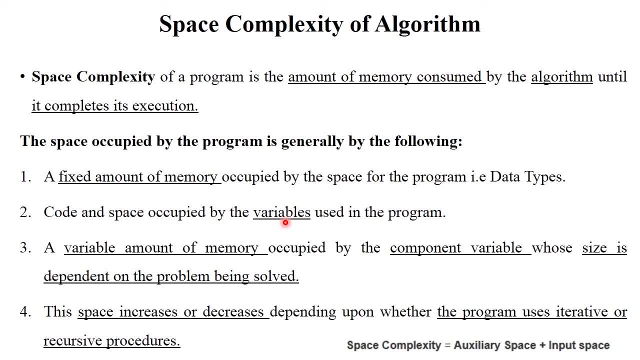 variable required the particular data type. So this is the one factor of space complexity. So this is the one factor of space complexity. Another code and space occupied by the variable in the program is given the name of the variable. It requires that particular space or memory. 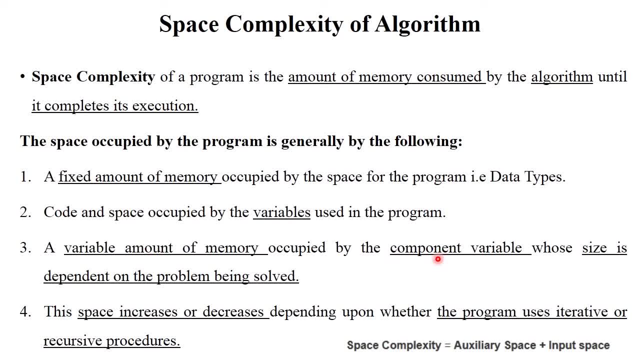 okay, Then also some variable amount of memory occupied by the component variable, whose size is dependent on problem being solved. Sometimes we have to declare a equal to 5 and after that we have to declare a equal to 10 on the same program. So it depends on your problem. 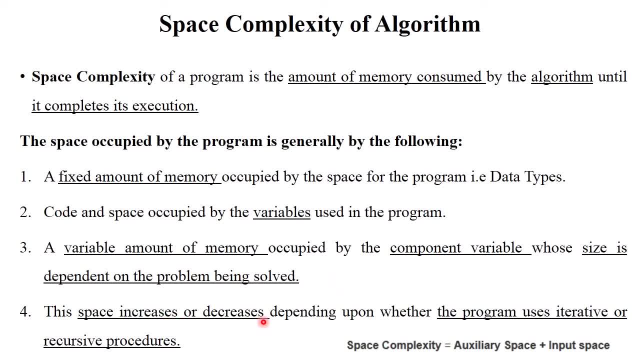 being solved okay. And also the space is increase or decrease. It is depending upon the program uses iterative or recursive procedure. I already explained in my previous video that video recursive function or recursive procedure. so this procedure also required a particular memory or particular space clear. so these are the factors where space complexity is depend. 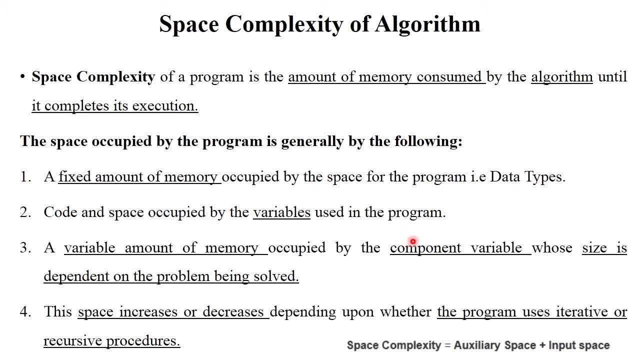 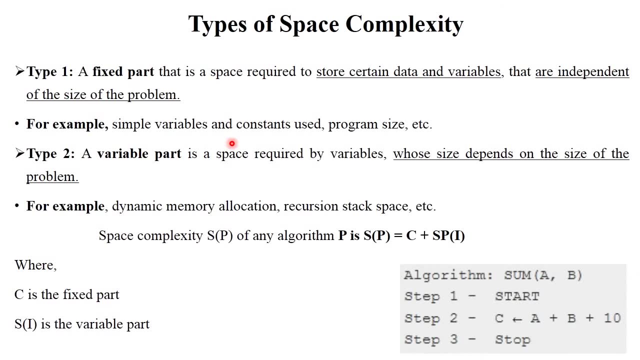 which includes data types, variables, component variables, recursive function. those all things require the particular space in memory. okay, so auxiliary space plus input space is called as space complexity clear next. so types of space complexity: generally there are two types: fixed part and variable part. fixed part: that is space required to store the certain data and variables. 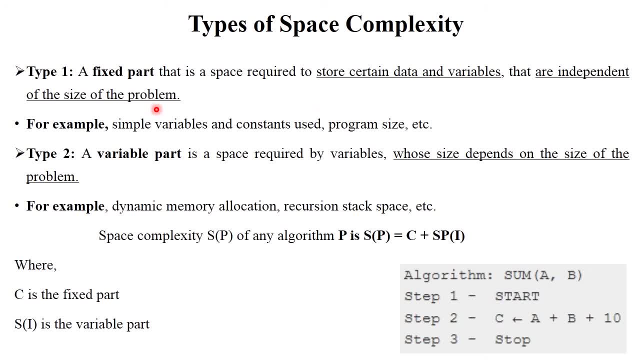 these are the independent size of the problem or constant part. okay, and the examples of fixed part is simple: variable and constants that used are also a program size. and the next type is variable part. variable means continuously change. this space is required by the variables whose size depend on the size of the problem. see here: this is just example where algorithm is sum. 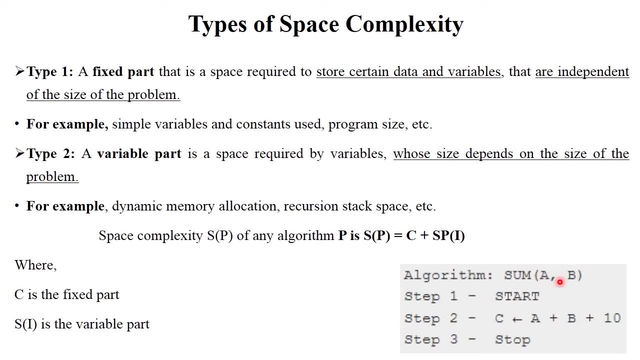 we have to pass two parameters, that is a and b, now algorithm start and algorithm stop, and in between that a plus b plus 10, and all the results or values are stored into the c. okay. so here 10 is a constant part, okay, and a and b is the variable part. sometime we have to pass 5 plus 3, sometimes again we have to. 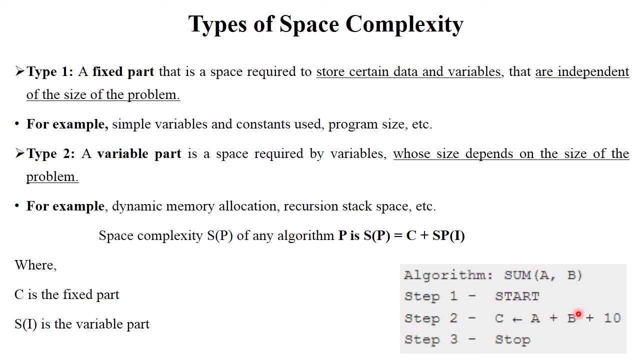 pass 10 plus 5. so a and b is not a constant value. it can be changed as per the requirement, clear. so a plus b, these are the variable part and 10 is fixed part. so it stored their space into this fixed part and a plus b stored their memory space into the variable part clear and result is again stored. 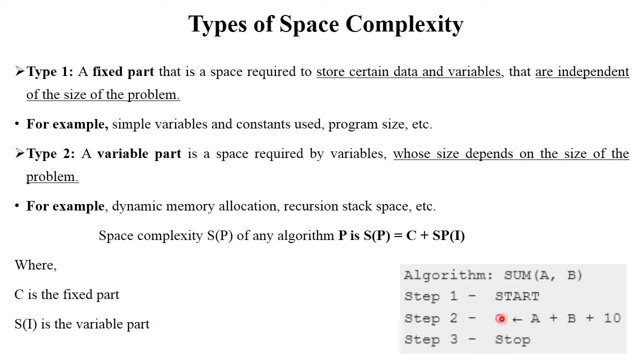 into the c. this is also a variable part, clear. so the space complexity of algorithm is sp, that is space complexity of that particular program. okay, s means space, p means program equal to variable part plus constants part. constant part is declared as a c, that is 10 and sp of i. sp of i means variable. 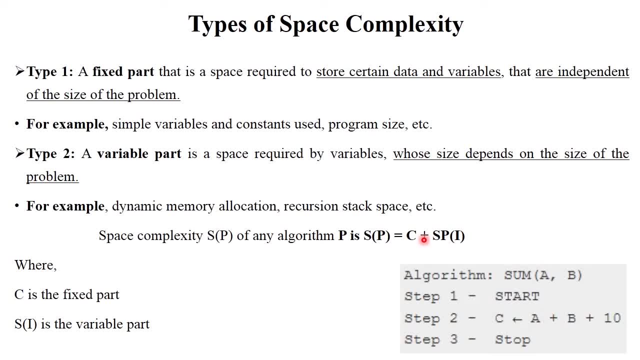 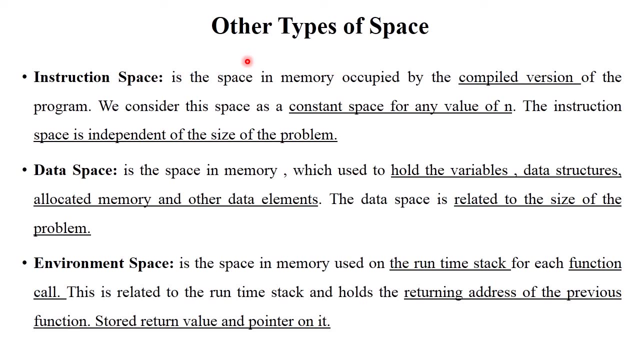 part. okay, these are the variable part, so constant plus variable part equal to space complexity. clear, this is the types of space complexity. next now there are again other types of space of memory in your program or in your computer: instruction space, data space and environment space. instruction space is the space of memory occupied by compile version of the 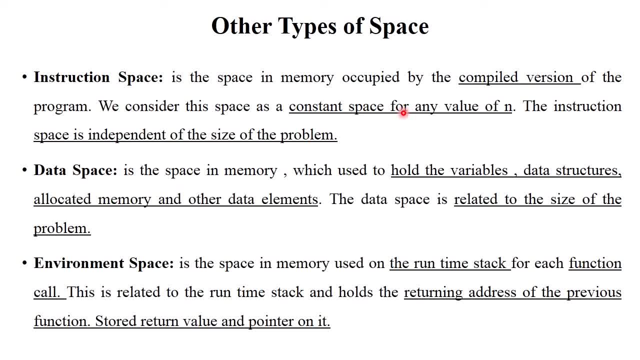 program. when you compile the particular program, some value or some part is constant part. okay, so. ok, so we consider this space as a constant space, that is, evaluation or labor spaceed portion. okay, so this means that the x plus x is constant. okay. so, in other words, the first standard part of this one is our ordinary parts. of it and that is called the velocity matrix. and because x equals to a, this means the value of k. it means that there is no space in the BiennialExperience space. that is the basic value if any other parts that is significant less than zero. and then, and comes the text for chickens. 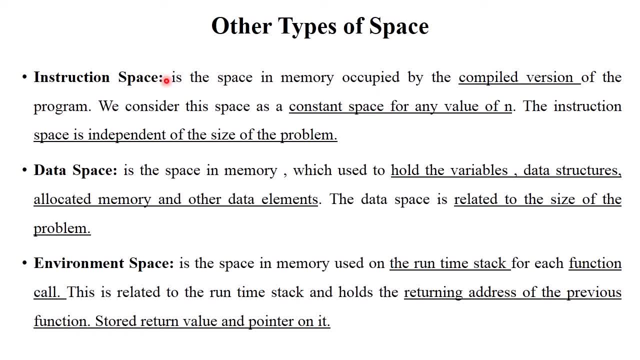 in terms of this, we would have to consider the order and then, for sofort, we would need two things to do here: filled and value of n, so our constant value, are stored into the instruction space. for example, pi equal to 3.4, okay, 3.14. so this is the constant value. our constant value are stored into the instruction. 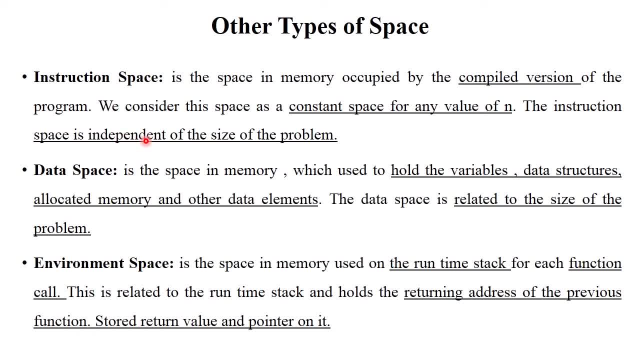 space. the instruction space is independent. it does not depends on each other. okay, so this is called as instruction space. the next one is data space. data space means which used to hold the variables, data structures, allocated memory and other data elements. you have to declare many variables in your program, like integer a, integer b, float c, etc. and also data structures like stack. 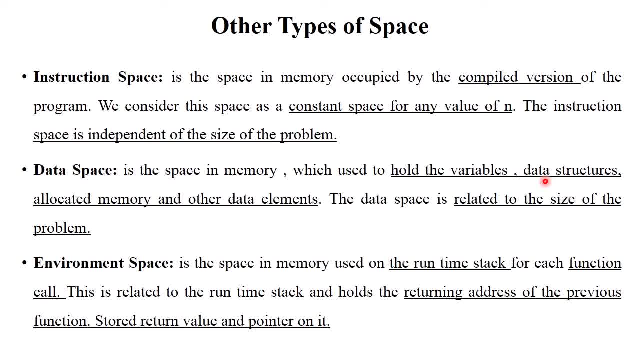 queue link list. you have to use this kind of data structures while implementation. so this: all data is stored into the data space. okay, the data space is related to the size of the problem. it continuously change as per the requirement. okay, and the last one is environment space. 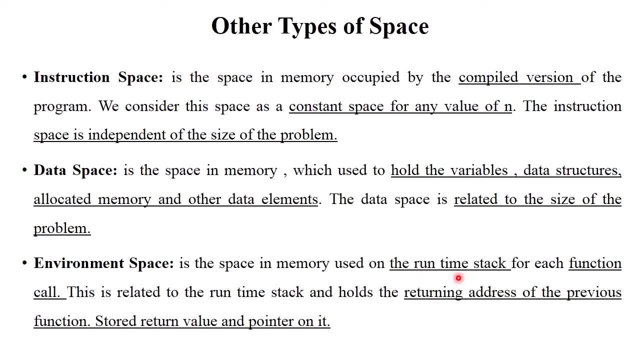 environment space is a memory used to runtime stack for each function call. when you call the particular function this kind of memory, it can be stored into the environment space. this is related to the runtime stack and hold a returning address of previous function, for example, recursive function. it. 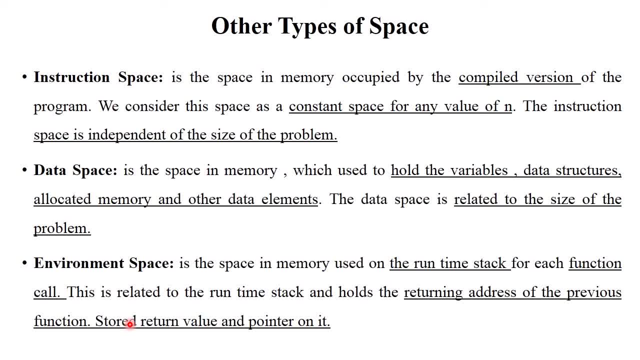 function calling itself. this is called recursive function and all this kind of memory are stored into the environment space. it stored the return value and pointer on it clear. for example, we have to perform a plus B, equal to C, so stored all the value into the C. this is called environment space clear. so these are the 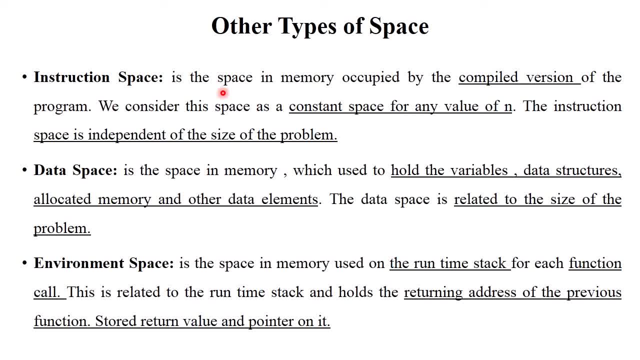 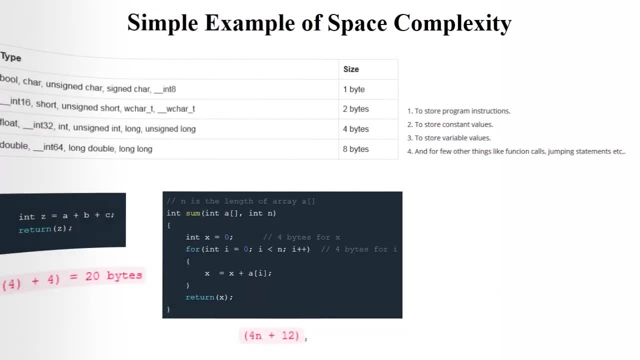 type of space: instruction space stored compiled versions or constant value. database stored variables, data structures and other some memory environment space is stored. all the recursive function returning address and pointers value clear next. now, this is a simple example of space complexity. we know that each and every data types required some constant size. for example, you have to use integer. 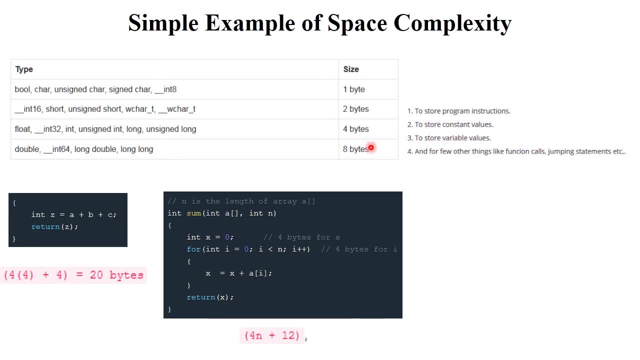 variable like integer a, so it requires 4 bytes of size in memory. ok, now see here integer Z, equal to a plus B plus C. so a, this variable required 4 bytes, B required 4 bytes and C also required 4 bytes- 4 plus 4, 8, 8 plus 4. 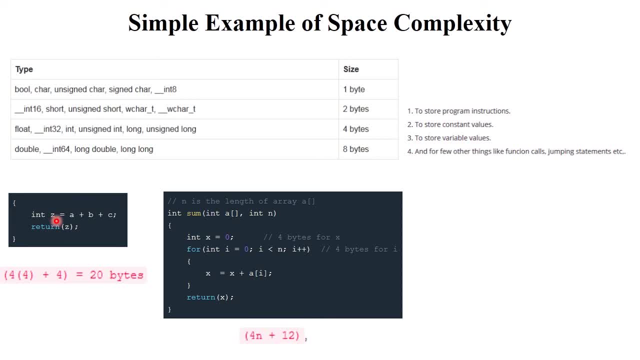 plus 12 and all this value are stored into the Z, that is again 4 bytes is required for solution. that is 4 plus 4 plus 4 and again plus 4, that is 16 bytes is required, ok, and after that the return Z is: 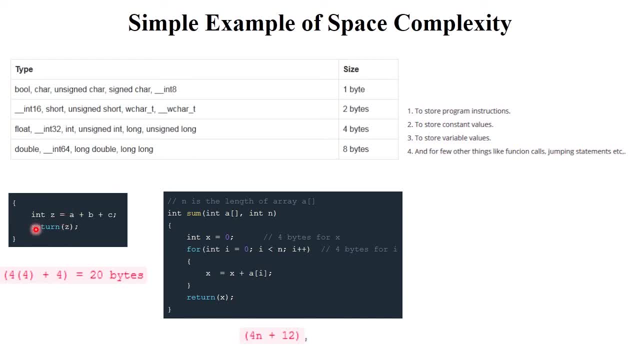 answer is return for printing purpose. so this again required 4 bytes of size in environment space. ok, so total required 20 bytes of space for this calculation clear. similarly in this example, see here: integer x equal to 0, integer i equal to 0 and integer n- these are the constant value, okay, and these are all are integer type, so integer. 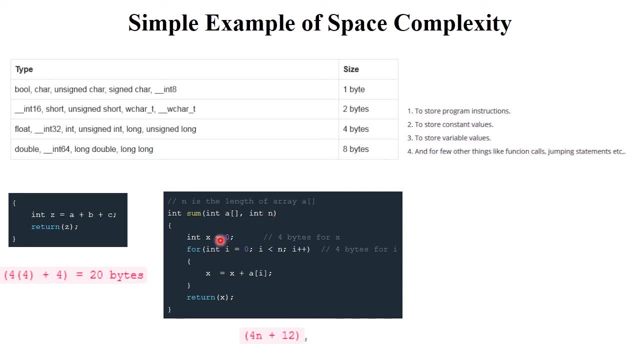 required always 4 bytes of size, so 4 plus 4 and plus 4. it requires total 12, clear, and after that, that is this for loop is executed up to n times, okay, and these all are integer variables. so it's required for n means for n plus 12. this kind of size is required for this execution of.